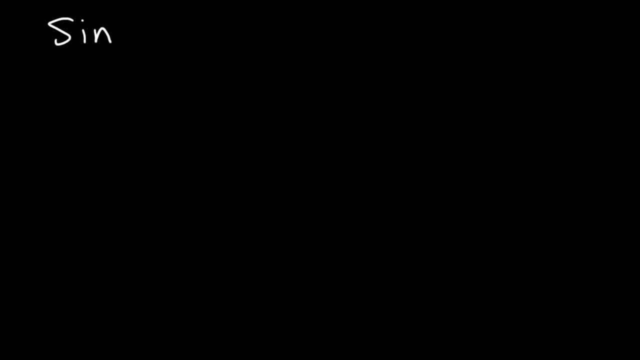 Consider this equation: sine x is equal to one half. What is the value of x? So sine of what angle is equal to one half. If you use the unit circle, you know that sine of 30 degrees, or pi over 6, is equal to one half And sine is positive in quadrants 1 and 2.. 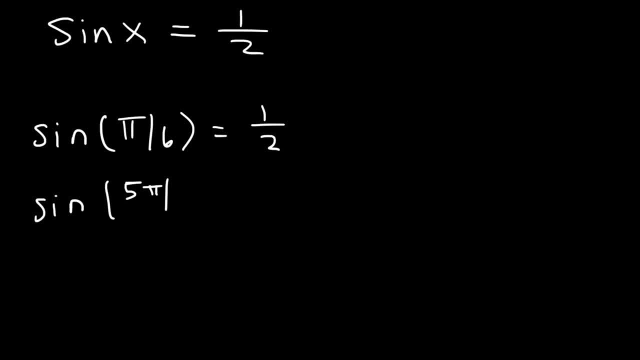 So sine 5 pi over 6 is also equal to one half. So therefore you can say x is equal to pi over 6 and x is equal to 5 pi over 6.. But if you want to find all solutions, it doesn't end there. 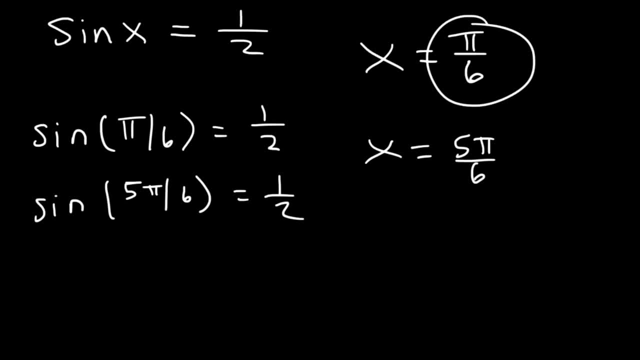 For example, if you add 2 pi to pi over 6, that would give you 13 pi over 6.. Sine of 13 pi over 6 is also one half. And if you add 2 pi to 5 pi over 6, that will give you another cool terminal angle. 2 pi is the same as 12 pi over 6.. So 5 pi over 6 plus 12 pi over 6 is 17 pi over 6.. 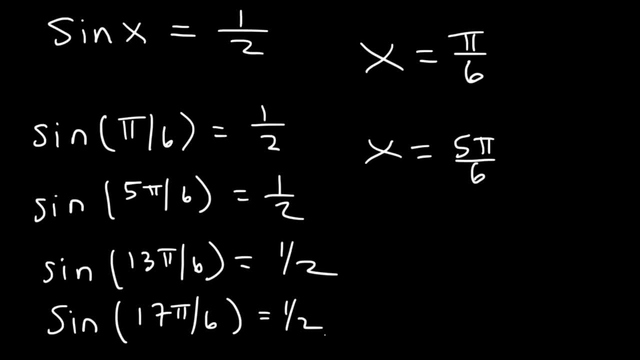 So to write an equation that gives us all solutions, it's going to be pi over 6 plus 2 pi n. The period of sine and cosine is 2 pi Where n is any integer. So n could be 0, plus or minus 1, plus or minus 2,, and so forth. 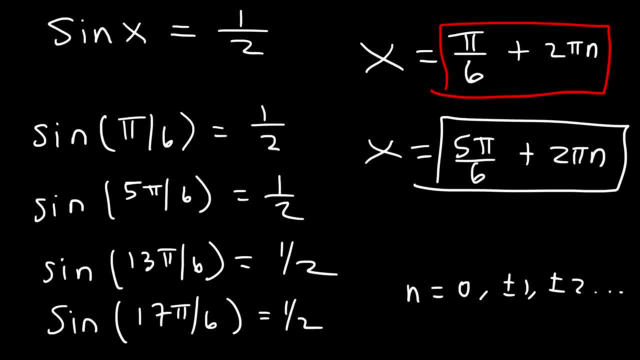 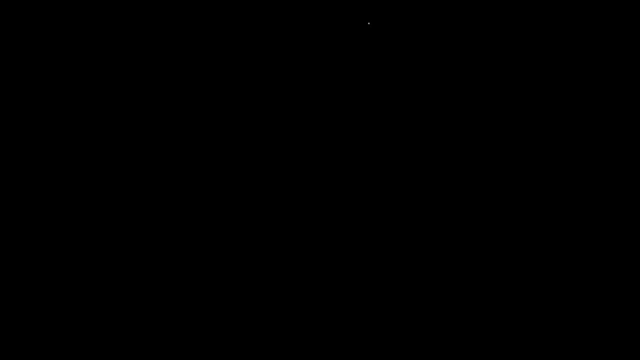 And so these are the two answers. So anytime you need to find all solutions, make sure you write your answer in terms of n. Let's work on another example. So let's say that cosine x Is equal to negative square root 2 divided by 2.. 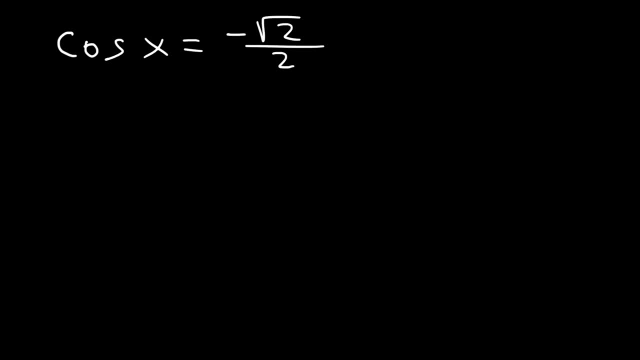 Find all answers that satisfies this equation. So cosine of what angle is equal to negative square root 2 over 2?. Now keep in mind: cosine is negative in quadrants 2 and 3. And you need to know the reference angle. 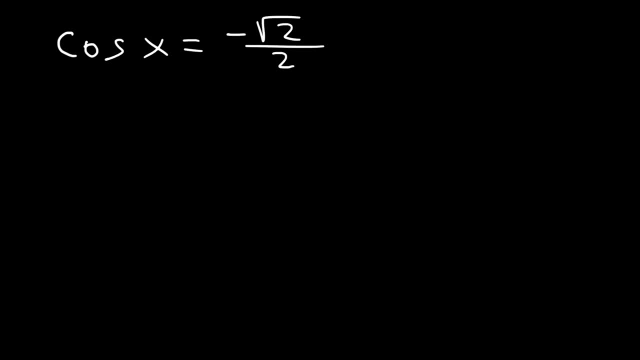 Find all answers that satisfies this equation. So cosine of what angle is equal to negative square root 2 over 2?. Now keep in mind: cosine is negative in quadrants 2 and 3. And you need to know the reference angle. 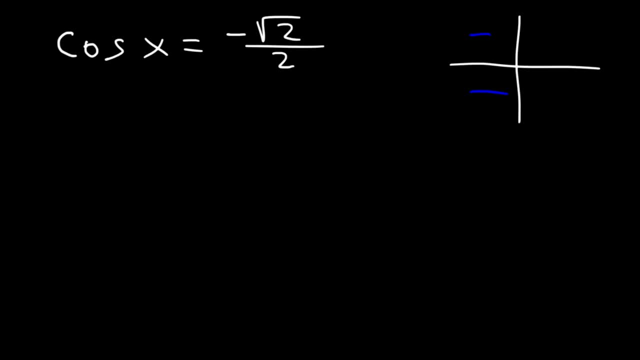 Cosine 45 is equal to the square root of 2 over 2.. So in quadrant 2.. In quadrant 2. An angle of 135 produces a reference angle of 45.. And in quadrant 3. 225 produces a reference angle of 45.. 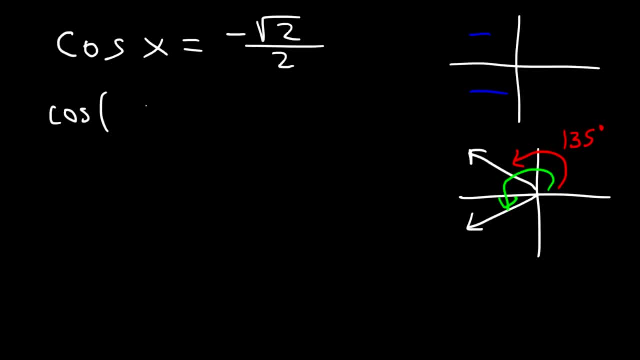 So therefore, cosine of 135 degrees, or cosine 3- pi over 4. That's equal to negative square root 2 over 2. And also cosine 5- pi over 4. It's equal to the same value. So we can write the solution as this: 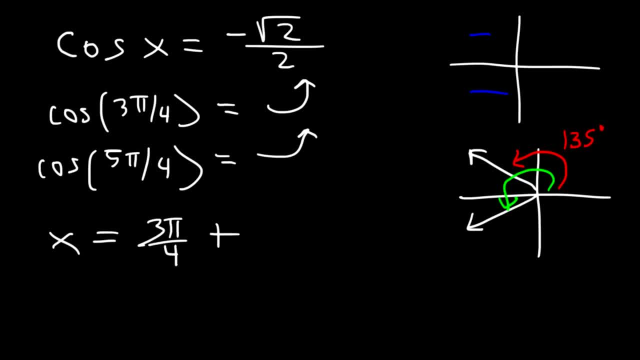 x is equal to 3 pi divided by 4 plus 2 pi n, Where n is any integer. And x is also equal to 5 pi over 4 plus 2 pi n. Here's another one. Let's say we have this equation: 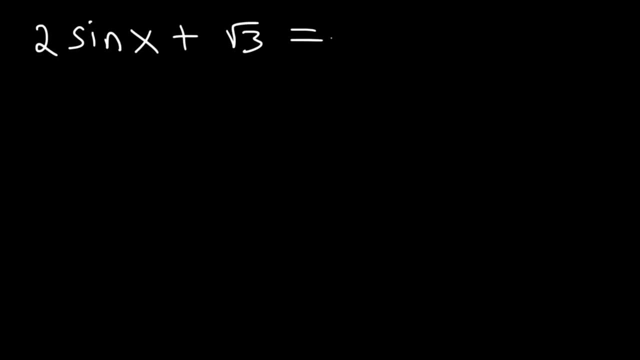 2 sine x plus the square root of 3.. Let's say it's equal to 0.. And this time we're going to restrict our answers from 0 to 2 pi. So when you see this, that means you don't need to add 2 pi n to your answer. 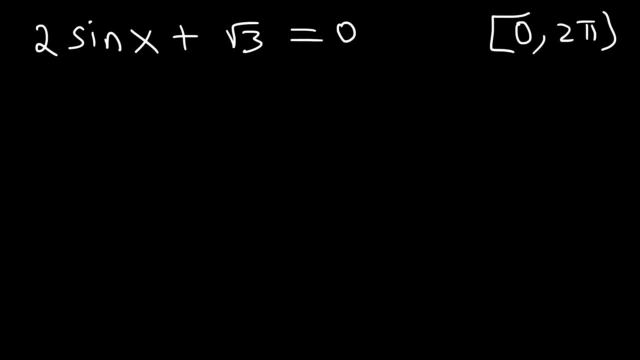 You only want the answers in this range. So first let's isolate sine x, And we could do so by subtracting both sides by the square root of 3.. So 2 sine x Is equal to negative square root 3.. 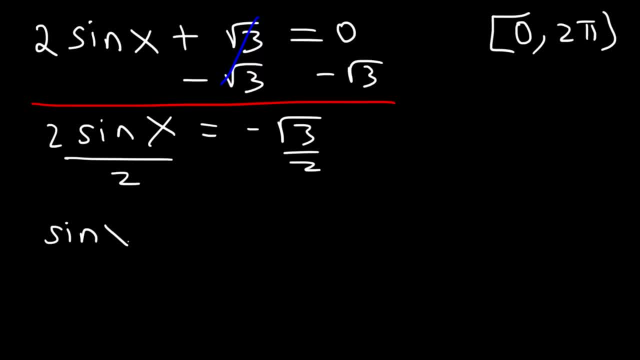 And now let's divide both sides by 2.. So sine x is equal to negative square root 3 over 2.. Now, first let's find a reference angle. If we draw the 30-60-90 triangle Across, the 30 is 1.. 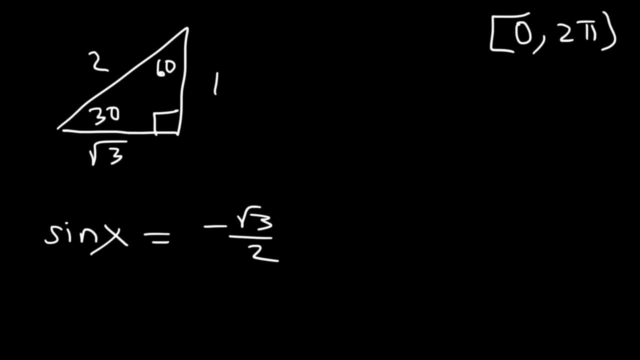 Across 60 is root 3. And across the hypotenuse, And the hypotenuse is 2.. Now the angle has to be 60. Because sine is equal to opposite, which is root 3. Divided by the hypotenuse. 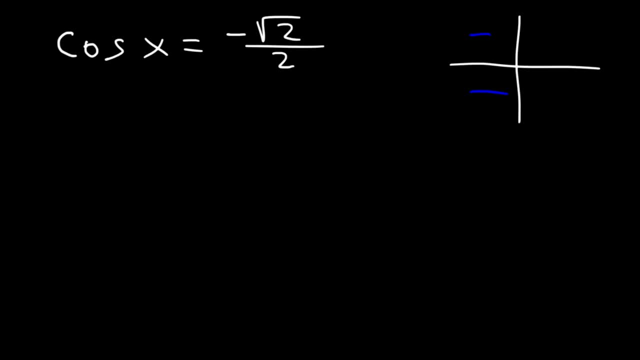 Cosine 45 is equal to the square root of 2 over 2.. So in quadrant 2.. In quadrant 2. An angle of 135 produces a reference angle of 45.. And in quadrant 3. 225 produces a reference angle of 45.. 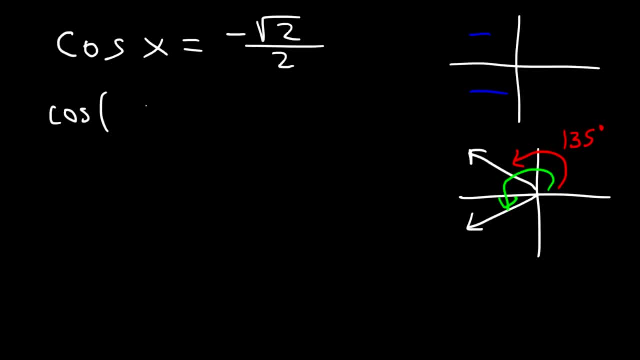 So therefore, cosine of 135 degrees, or cosine 3- pi over 4. That's equal to negative square root 2 over 2. And also cosine 5- pi over 4. It's equal to the same value. So we can write the solution as this: 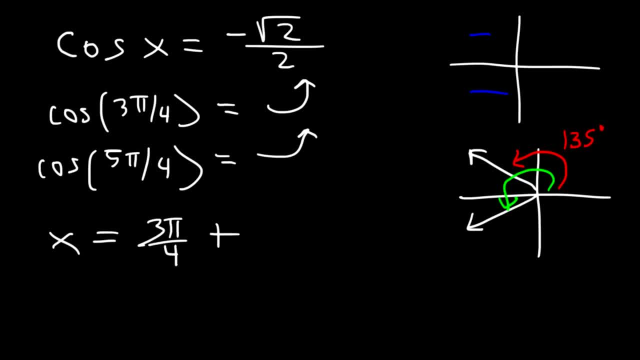 x is equal to 3 pi divided by 4 plus 2 pi n, Where n is any integer. And x is also equal to 5 pi over 4 plus 2 pi n. Here's another one. Let's say we have this equation: 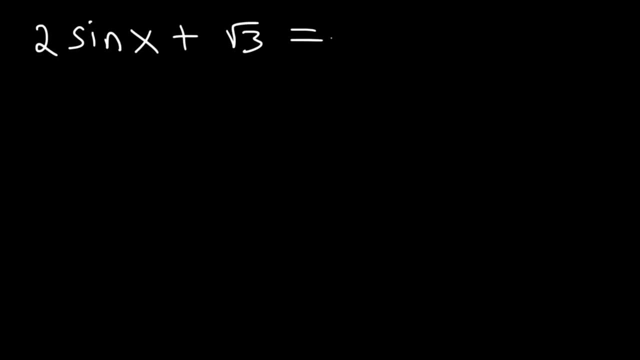 2 sine x plus the square root of 3.. Let's say it's equal to 0.. And this time we're going to restrict our answers from 0 to 2 pi. So when you see this, that means you don't need to add 2 pi n to your answer. 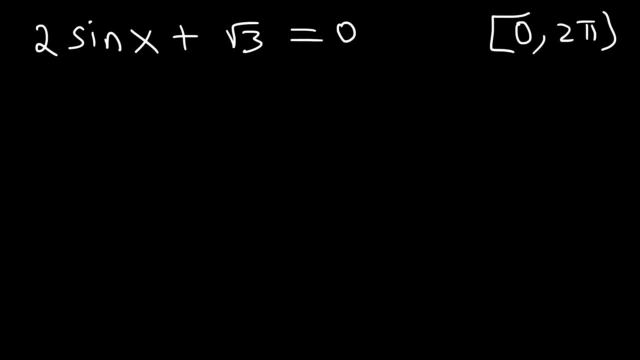 You only want the answers in this range. So first let's isolate sine x, And we could do so by subtracting both sides by the square root of 3.. So 2 sine x Is equal to negative square root 3.. 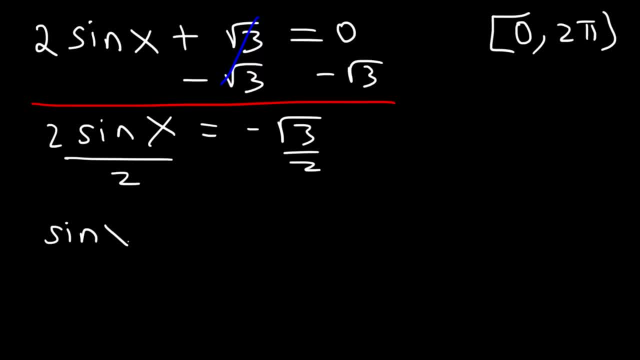 And now let's divide both sides by 2.. So sine x is equal to negative square root 3 over 2.. Now, first let's find a reference angle. If we draw the 30-60-90 triangle Across, the 30 is 1.. 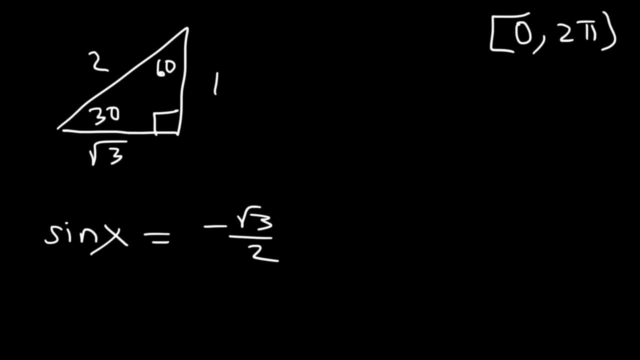 Across 60 is root 3. And across the hypotenuse, And the hypotenuse is 2.. Now the angle has to be 60. Because sine is equal to opposite, which is root 3. Divided by the hypotenuse. 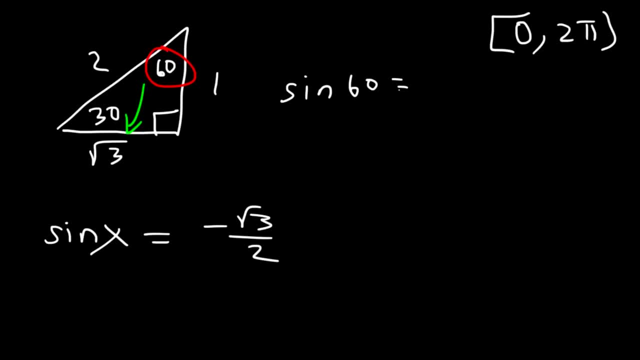 So we know that sine 60, or sine pi over 3, is equal to root 3 over 2.. But now we need the angle in quadrants 3 and 4.. That's where sine is negative. 240, or 4 pi over 3, has a reference angle of 60. 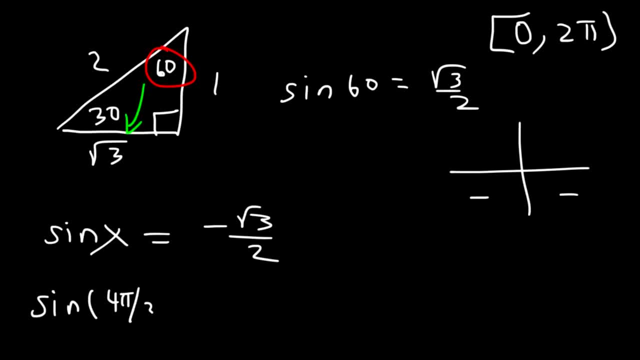 So sine of 4 pi over 3 is equal to this value, And also 5 pi over 3 have the same reference angle as pi over 3. And so that will give you that answer. So x is equal to the values inside. 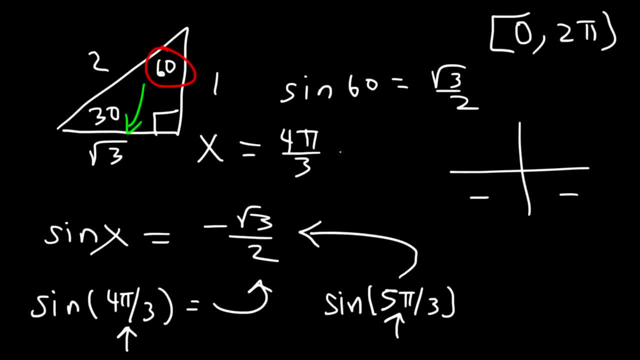 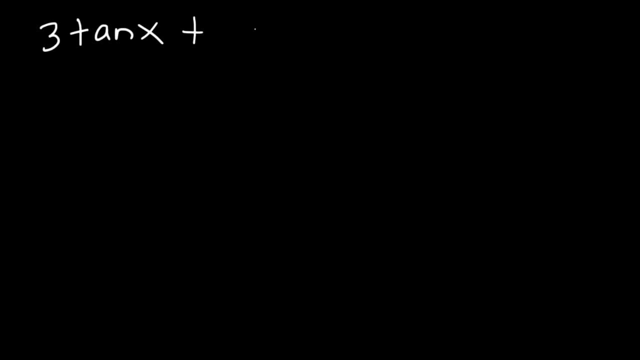 x is an angle. So x is 4 pi over 3 and 5 pi over 3.. Which is in this range. So these are the answers to this problem. Here's another one that you can try: 3 tangent x plus the square root of 3 is equal to 0.. 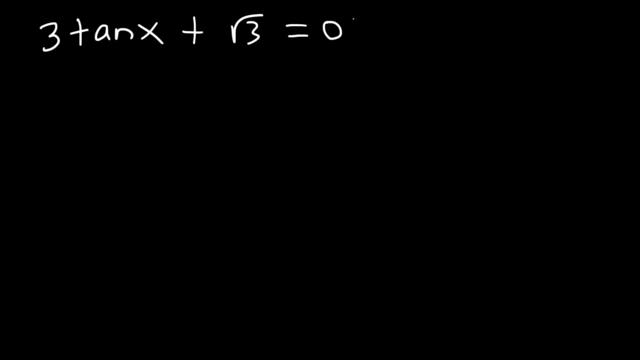 Find all solutions. So that means you want to write your answer with n. So what should we do? The first thing we need to do is subtract both sides by the square root of 3.. So 3 tan x is equal to negative root 3.. 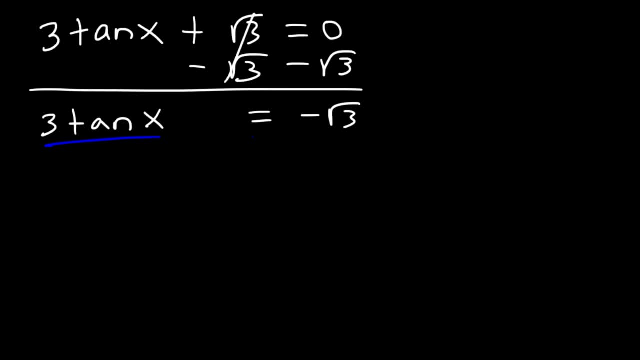 Next, let's divide both sides by 3.. So now we have this expression: Tangent x is equal to negative square root 3 divided by 3.. So what reference angle will give us this value If we draw the 30-60-90 triangle? 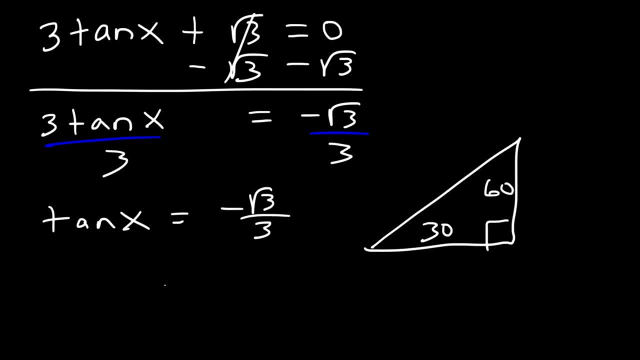 We need to use the 30 degree angle. Tangent of 30 is equal to the opposite side, 1 divided by the adjacent side, Now 1 over root 3, if you rationalize it is equivalent to the square root of 3 divided by 3.. 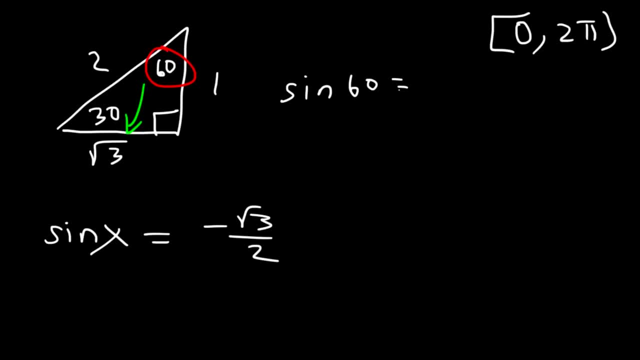 So we know that sine 60, or sine pi over 3, is equal to root 3 over 2.. But now we need the angle in quadrants 3 and 4.. That's where sine is negative. 240, or 4 pi over 3, has a reference angle of 60. 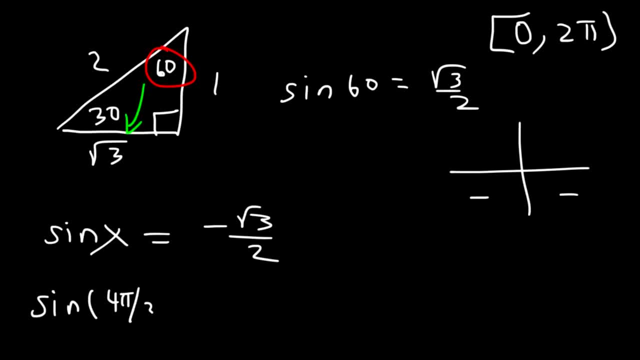 So sine of 4 pi over 3 is equal to this value, And also 5 pi over 3 have the same reference angle as pi over 3. And so that will give you that answer. So x is equal to the values inside. 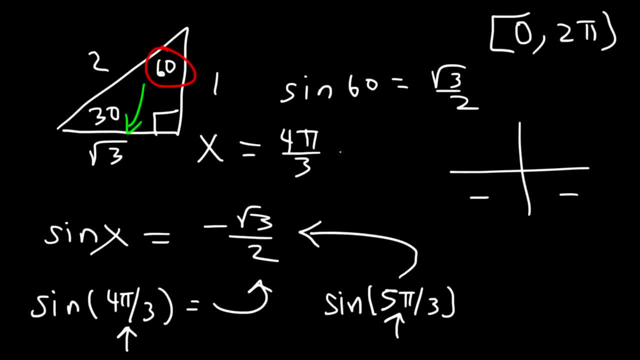 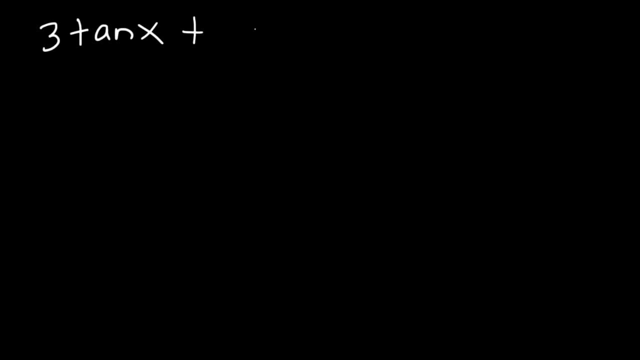 x is an angle. So x is 4 pi over 3 and 5 pi over 3.. Which is in this range. So these are the answers to this problem. Here's another one that you can try: 3 tangent x plus the square root of 3 is equal to 0.. 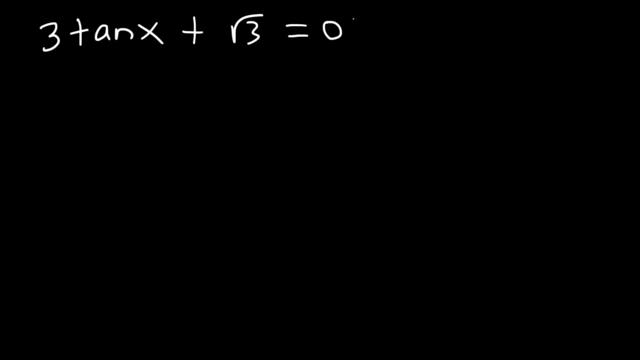 Find all solutions. So that means you want to write your answer with n. So what should we do? The first thing we need to do is subtract both sides by the square root of 3.. So 3 tan x is equal to negative root 3.. 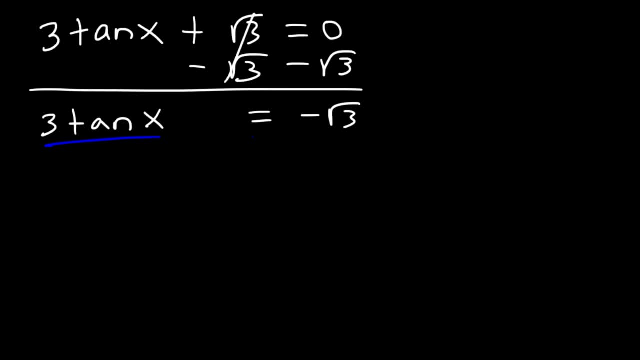 Next, let's divide both sides by 3.. So now we have this expression: Tangent x is equal to negative square root 3 divided by 3.. So what reference angle will give us this value If we draw the 30-60-90 triangle? 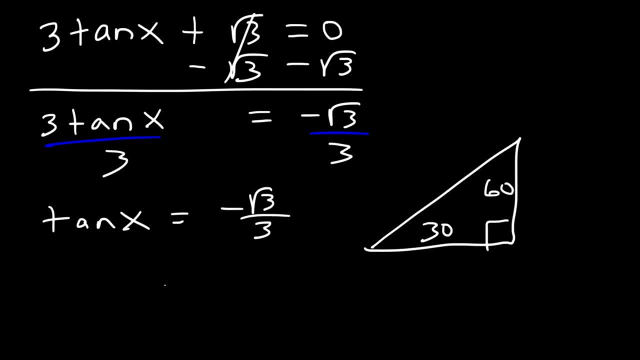 We need to use the 30 degree angle. Tangent of 30 is equal to the opposite side, 1 divided by the adjacent side, Now 1 over root 3, if you rationalize it is equivalent to the square root of 3 divided by 3.. 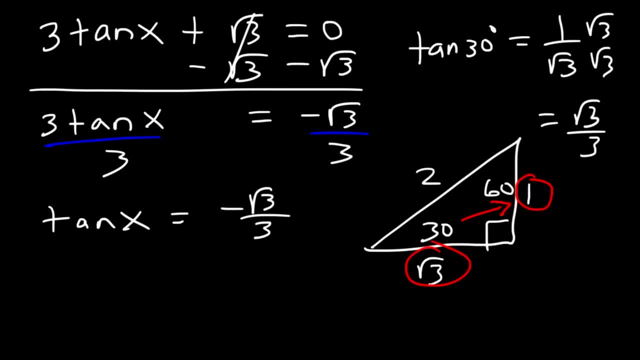 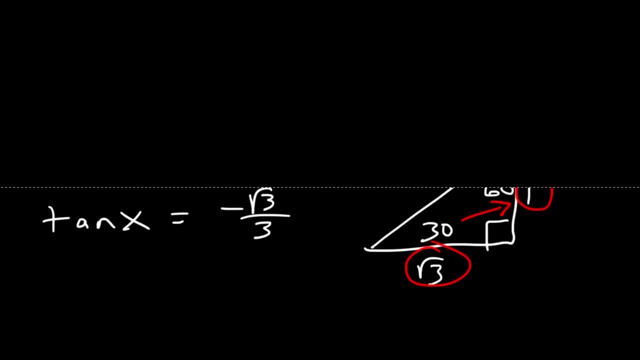 And so we have a reference angle of 30.. However, tangent is not negative in quadrant 1.. Tangent is negative in quadrant 2 and in quadrant 4.. So 150 will give us the angle in quadrant 2. And to get the angle in quadrant 4, that's 330. 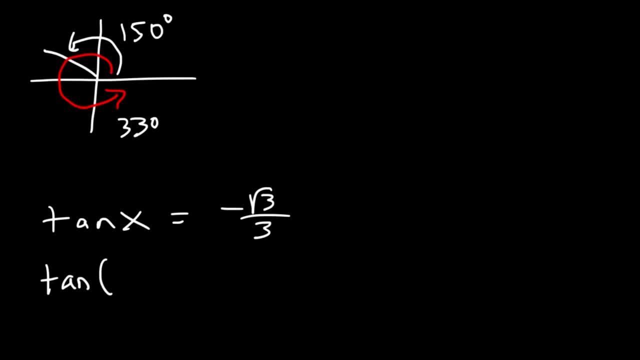 So tangent of 150,, which is the same as the angle in quadrant 2,, is the same as 5 pi over 6, is equal to negative square root 3 over 3.. And tangent 11 pi over 6,, which is 330,. 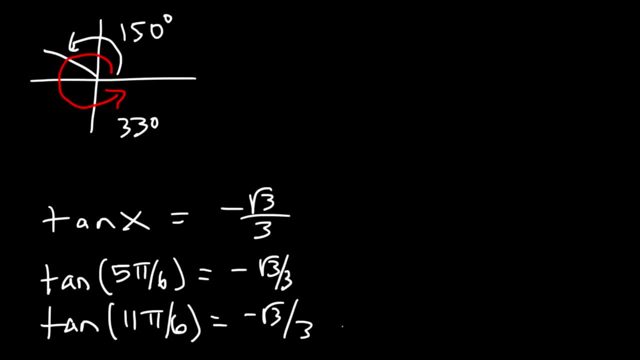 that's equal to the same thing. Now we said that the period of sine and cosine is 2 pi. The period of tangent and cotangent is pi. So to write the answers, you can write it like this: x is equal to 5 pi over 6 plus pi n, as opposed to 2 pi n. 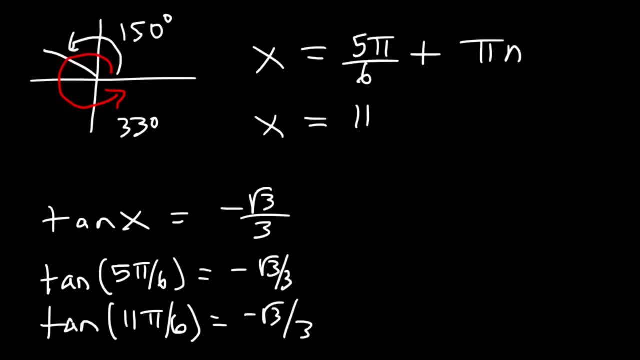 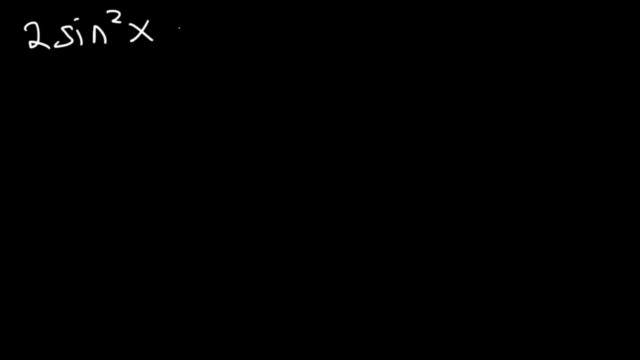 And it's also equal to 11 pi over 6 plus pi n, where n is any integer. And so these are the answers, And make sure to make some sort of statement that defines n. Here's another problem. Let's say that 2, sine squared, minus 1, is equal to 0.. 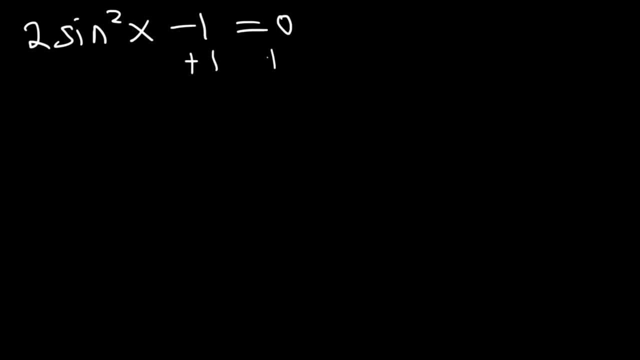 Let's find all solutions. So first we need to add 1 to both sides, And so 2 sine squared is equal to 1.. Next we need to divide both sides by 2. So sine squared is equal to 1 half. 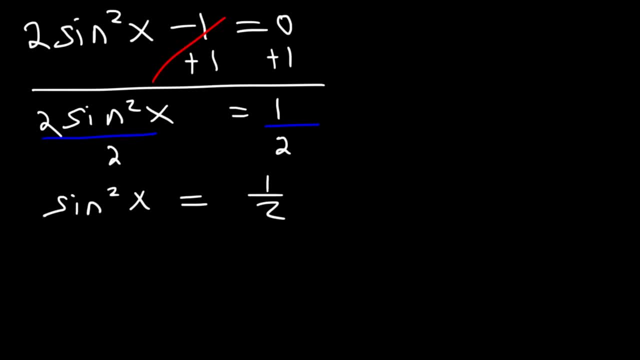 So now, what should we do at this point? The first step is to take the square root of both sides. The square root of sine squared is simply sine x. But now, what is the square root of 1? half The square root of 1 is 1.. 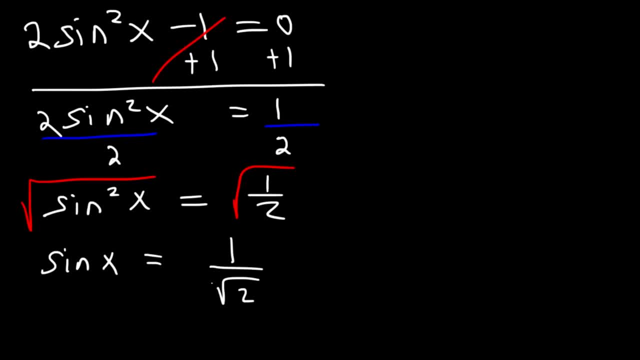 And the square root of 2 is the square root of 2. And it's going to be plus or minus, Because once you square something it's always going to be positive. For example, looking at the expression, sine squared is equal to 1 half. 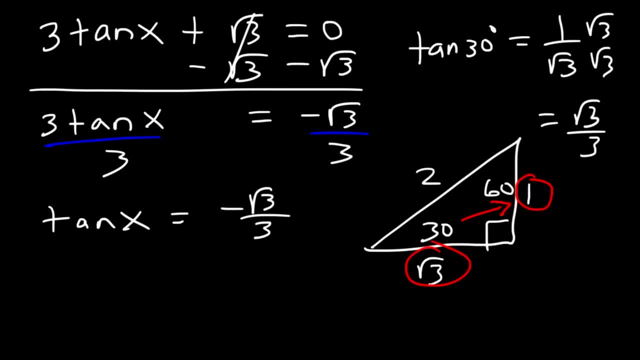 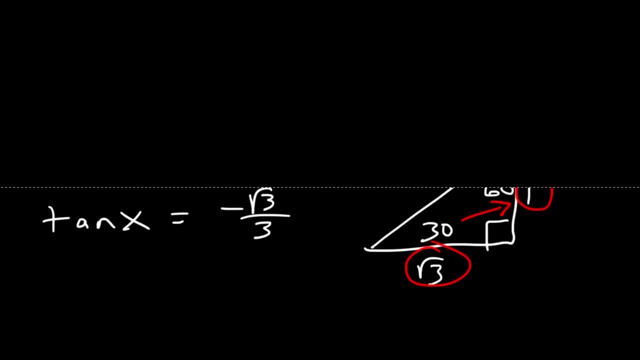 And so we have a reference angle of 30.. However, tangent is not negative in quadrant 1.. Tangent is negative in quadrant 2 and in quadrant 4.. So 150 will give us the angle in quadrant 2. And to get the angle in quadrant 4, that's 330. 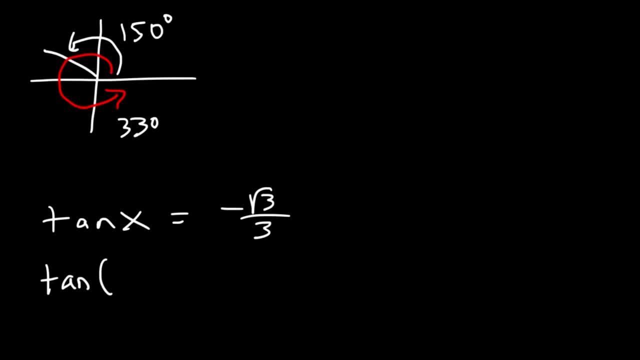 So tangent of 150,, which is the same as the angle in quadrant 2,, is the same as 5pi over 6, is equal to negative square root 3 over 3.. And tangent 11pi over 6,, which is 330,. 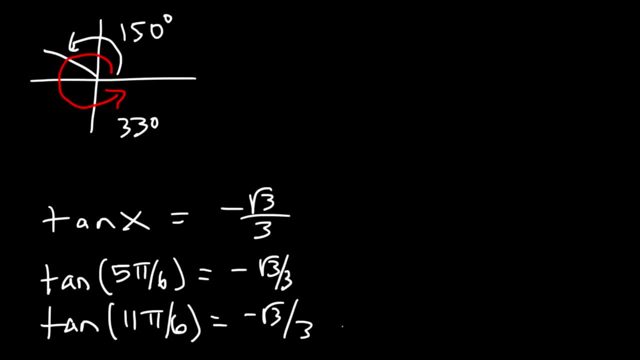 that's equal to the same thing. Now we said that the period of sine and cosine is 2pi, The period of tangent and cotangent is pi. So to write the answers, you can write it like this: x is equal to 5pi over 6 plus pi n, as opposed to 2pi n. 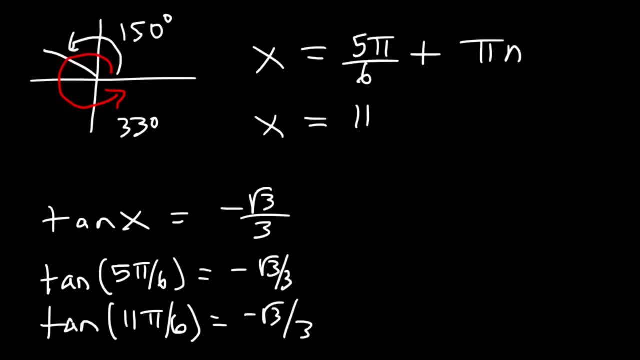 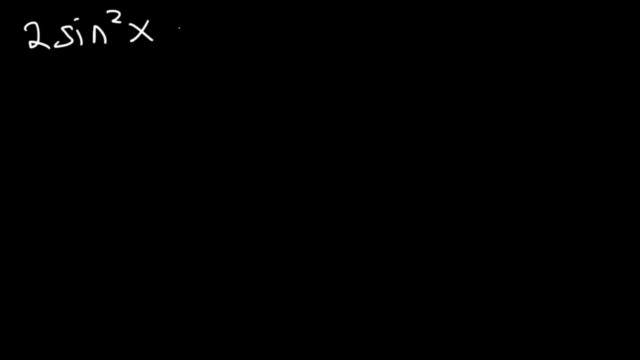 And it's also equal to 11pi over 6 plus pi n, where n is any integer. And so these are the answers, And make sure to make some sort of statement that defines n. Here's another problem. Let's say that 2, sine squared, minus 1, is equal to 0.. 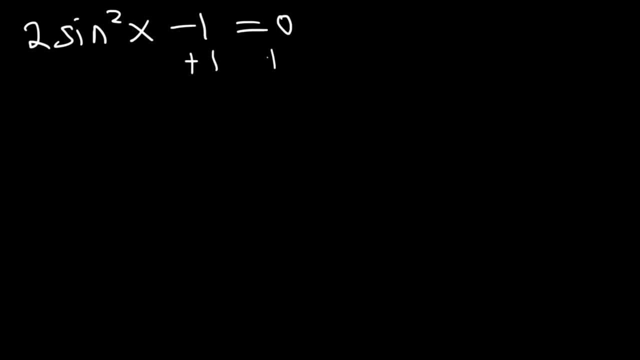 Let's find all solutions. So first we need to add 1 to both sides, And so 2 sine squared is equal to 1.. Next we need to divide both sides by 2. So sine squared is equal to 1 half. 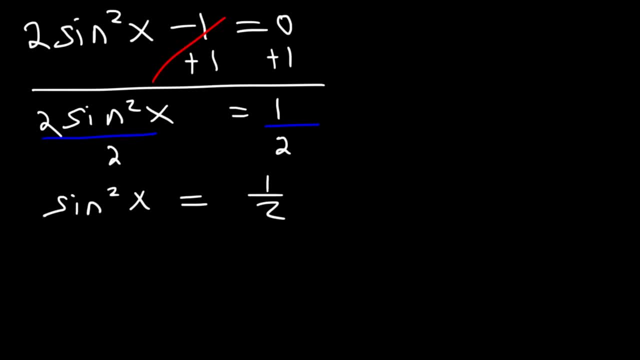 So now, what should we do at this point? The first step is to take the square root of both sides. The square root of sine squared is simply sine x. But now, what is the square root of 1? half The square root of 1 is 1.. 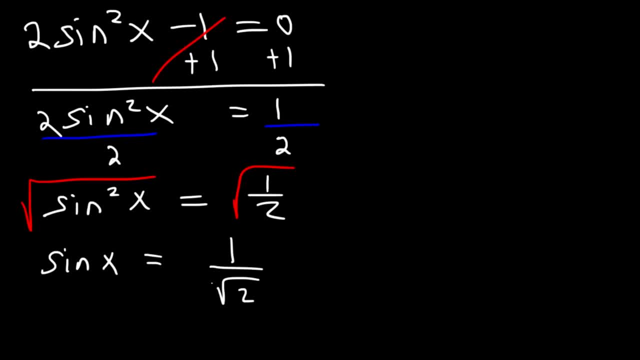 And the square root of 2 is the square root of 2. And it's going to be plus or minus, Because once you square something it's always going to be positive. For example, looking at the expression, sine squared is equal to 1 half. 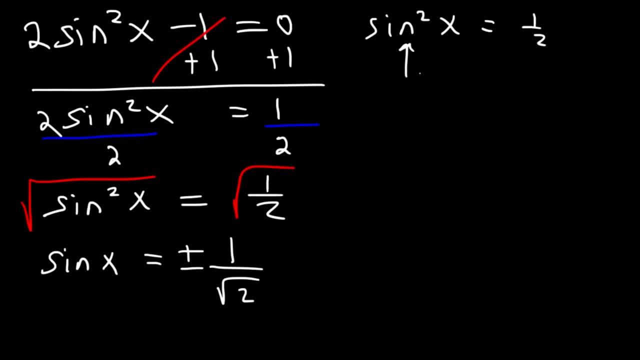 if I plug in positive 1 over square root 2 or negative 1 over square root over 2, it would still give me positive 1 half, Because when you square a positive number or a negative number, it will give you a positive result. 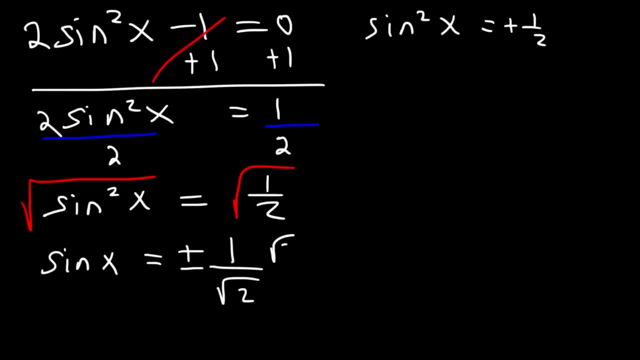 But now let's simplify: 1 over root 2. What we can do is rationalize it. So what we have now is plus or minus the square root of 2 divided by 2. So sine x can equal positive root 2 over 2 or negative. 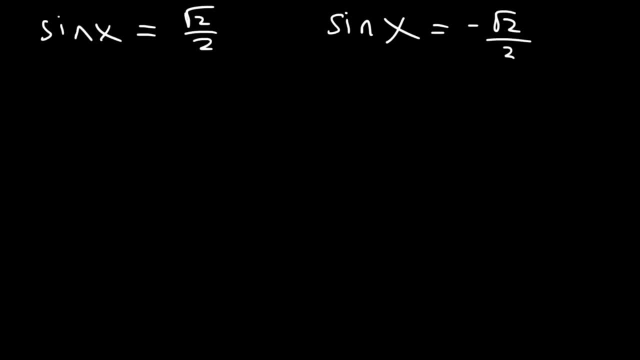 So therefore, instead of having two quadrants, the answer lies in all four quadrants. So sine is positive in quadrants 1 and 2.. So therefore, x could be 45 degrees or pi over 4.. And it could be 3 pi over 4.. 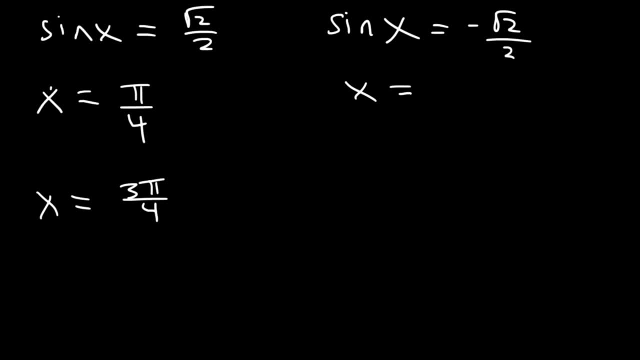 Now, sine is negative in quadrants 3 and 4.. So it could be 5 pi over 4 and 7 pi over 4.. Now to write an expression: to get all solutions we need to add 2 pi n to every answer. 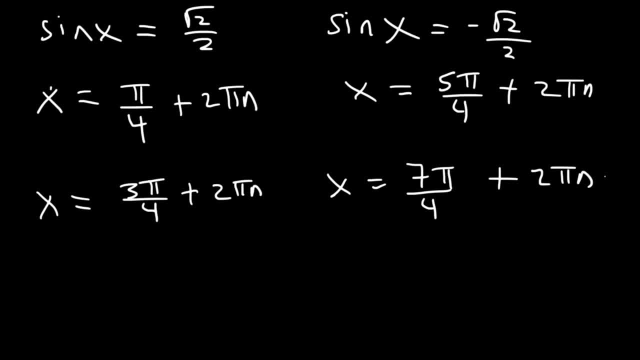 So you can write your answer like this if you want to. Now you can simplify this, since we have all four answers. Notice that each of these answers differ by pi over 2.. Pi over 4,, which is 45, differs from 3 pi over 4 by 90 degrees. 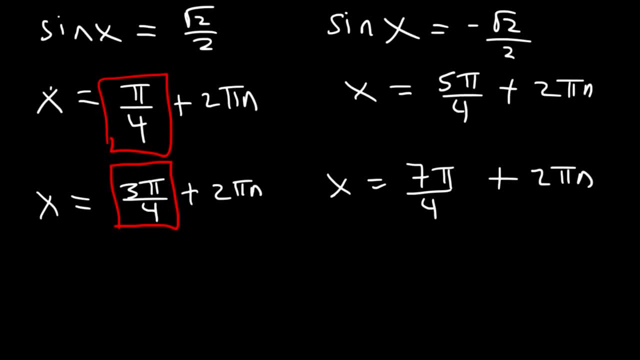 135 minus 45 is 90.. And if you add 90 to 135, you're going to get 225.. If you add 90 to 225, you get 315.. And so, because each of these answers differ by 90 degrees, 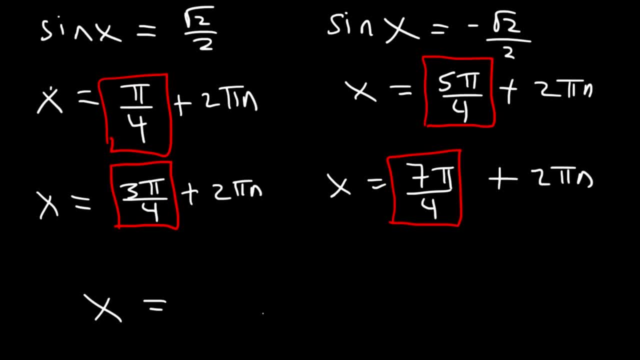 we can write one statement that represents all of these solutions. So we can write pi over 4, plus pi over 2, n Where n is any integer. So this will give us any answer. If n is 0, then we're just going to get pi over 4.. 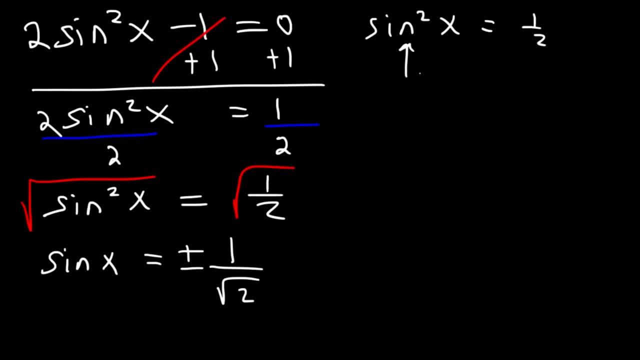 if I plug in positive 1 over square root 2 or negative 1 over square root over 2, it would still give me positive 1 half, Because when you square a positive number or a negative number, it will give you a positive result. 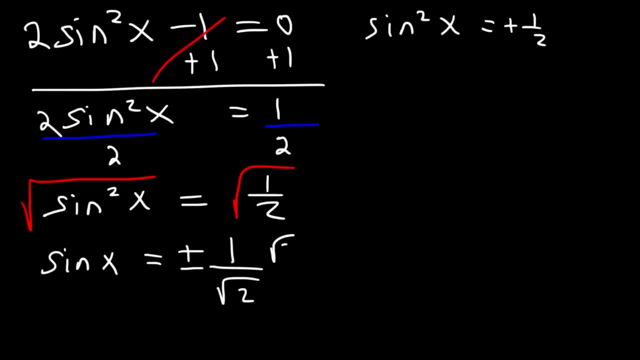 But now let's simplify: 1 over root 2. What we can do is rationalize it. So what we have now is plus or minus the square root of 2 divided by 2. So sine x can equal positive root 2 over 2 or negative. 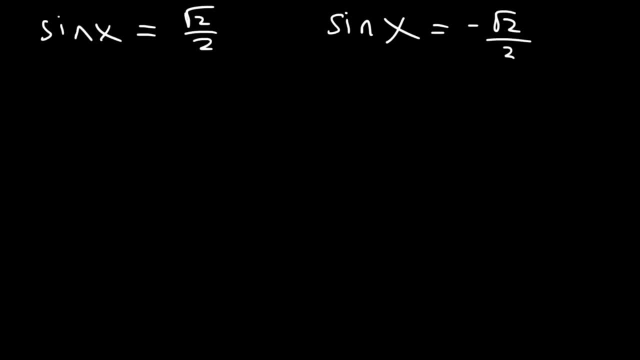 So therefore, instead of having two quadrants, the answer lies in all four quadrants. So sine is positive in quadrants 1 and 2.. So therefore, x could be 45 degrees or pi over 4.. And it could be 3 pi over 4.. 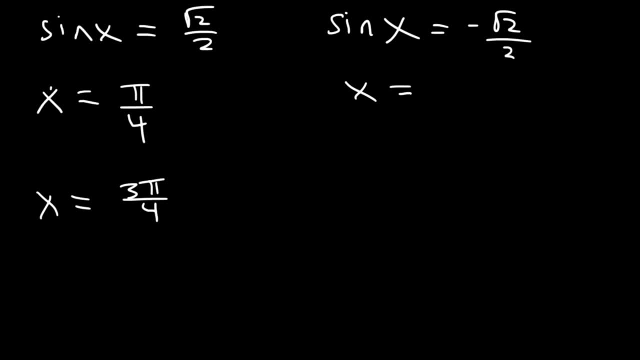 Now, sine is negative in quadrants 3 and 4.. So it could be 5 pi over 4 and 7 pi over 4.. Now to write an expression: to get all solutions we need to add 2 pi n to every answer. 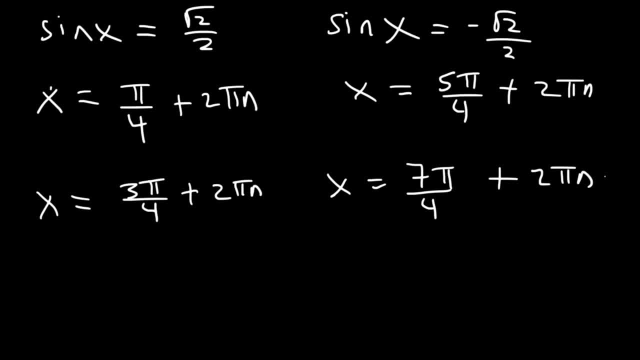 So you can write your answer like this if you want to. Now you can simplify this, since we have all four answers. Notice that each of these answers differ by pi over 2.. Pi over 4,, which is 45, differs from 3 pi over 4 by 90 degrees. 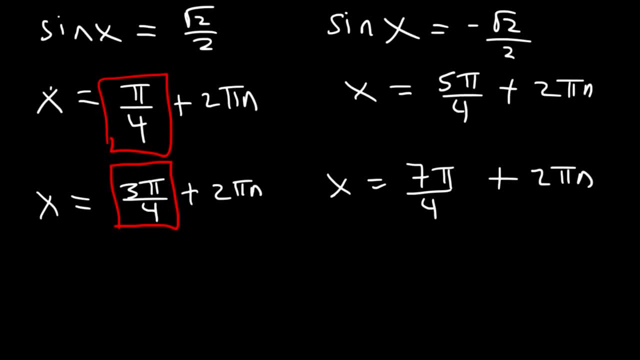 135 minus 45 is 90.. And if you add 90 to 135, you're going to get 225.. If you add 90 to 225, you get 315.. And so, because each of these answers differ by 90 degrees, 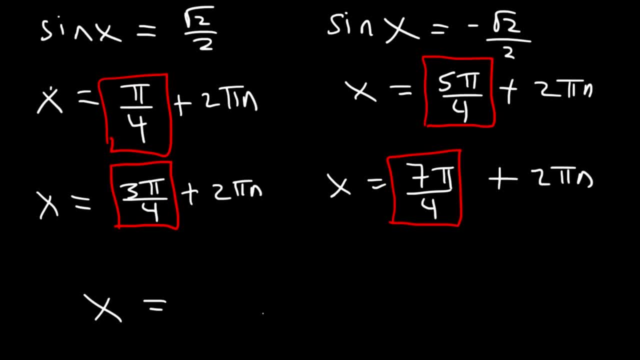 we can write one statement that represents all of these solutions. So we can write pi over 4, plus pi over 2, n Where n is any integer. So this will give us any answer. If n is 0, then we're just going to get pi over 4..